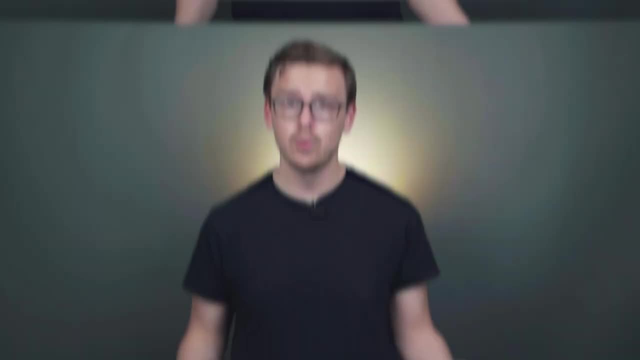 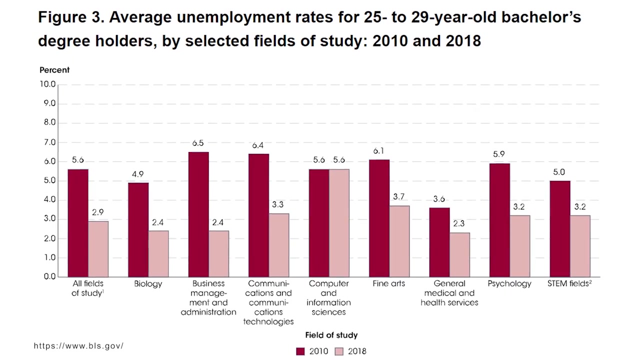 in the middle, but it's definitely above average when it comes to your salary. Now, one career path you might go down is becoming a chemist, of course, and they make around $78,000 a year. Now, if you look at the median annual earnings for young people, people between the ages of 25 and 29- for 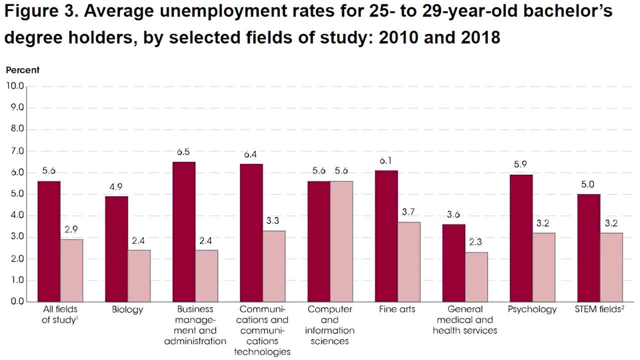 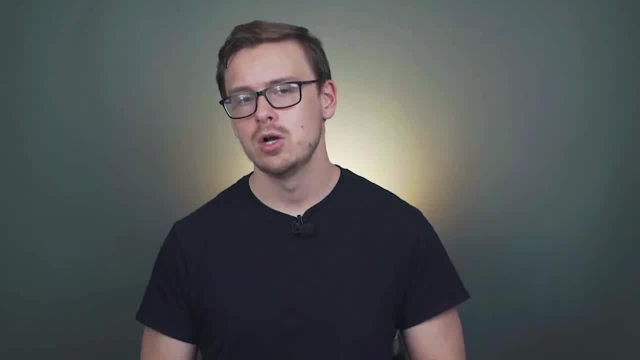 all different types of degrees, you see that STEM degrees tend to rank pretty well. So not only do you make more money down the line, but you also make more money right off the bat, at the beginning of your career. Overall, this one's 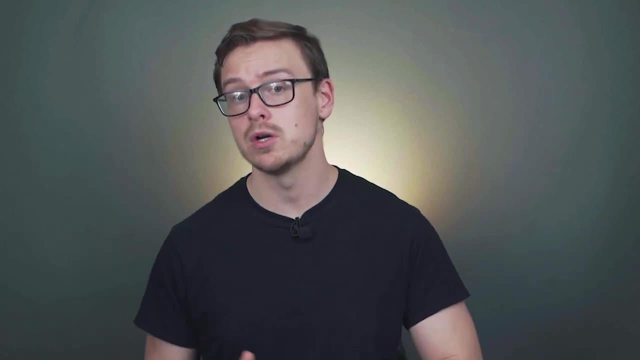 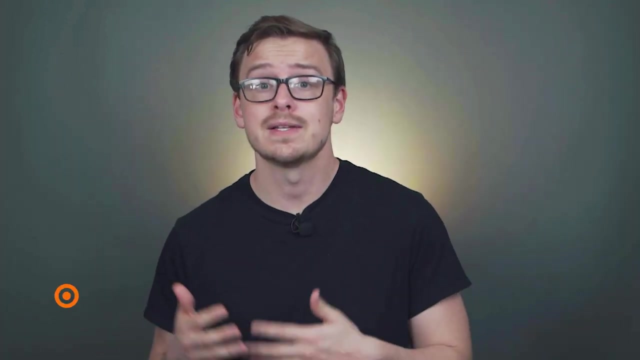 pretty good when it comes to science degrees and above average when you compare it to all degrees, So I'm going to give this one a 7 out of 10 when it comes to salary or earnings potential. Next we're going to be talking about satisfaction, and first we're going to go over meaning, which is: 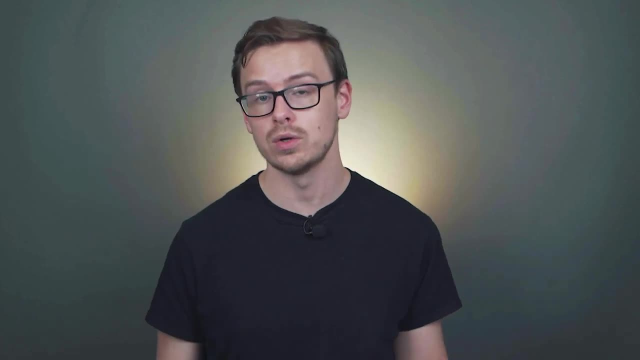 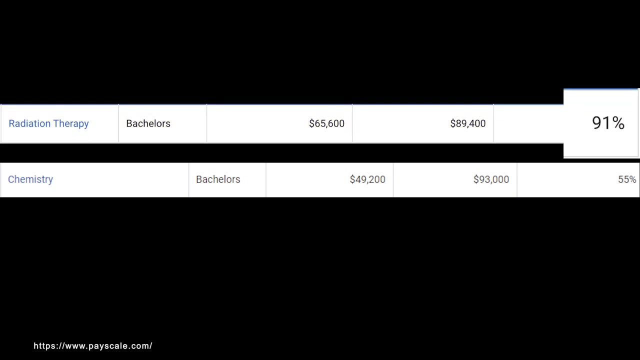 how much your career positively affects the rest of the world. So, when it comes to meaning, chemistry comes in at 55%, and you can compare that to radiation therapy at 91%, which is the highest, and one of the lowest is plastics engineering technology at 31%. So it's right there in the 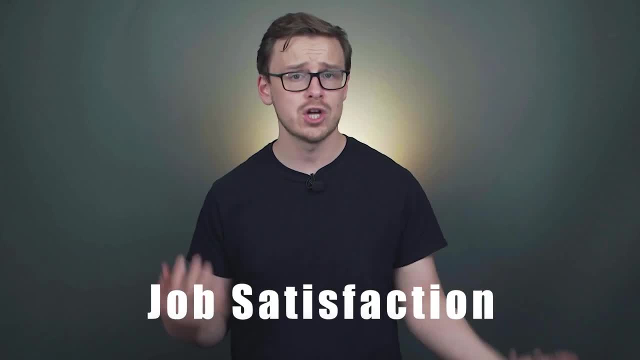 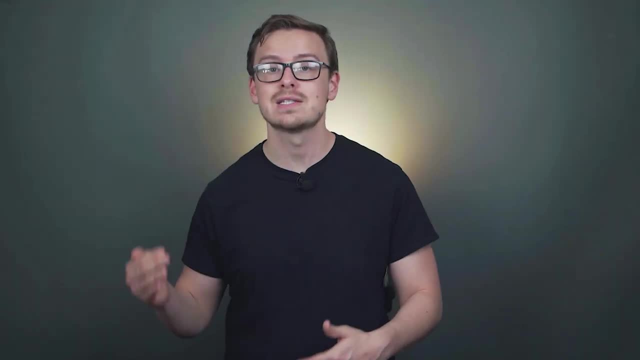 middle. I would say it's slightly above average. If you look at job satisfaction for something like material scientists, you'd see that it comes in at about 67%, which again is slightly above average as well. Now, science degrees tend to be some of the most regretted degrees. They're the second. 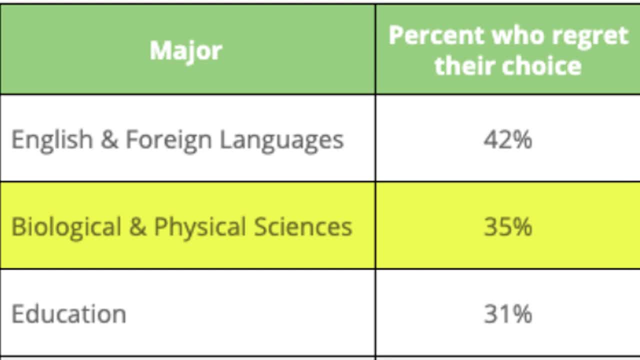 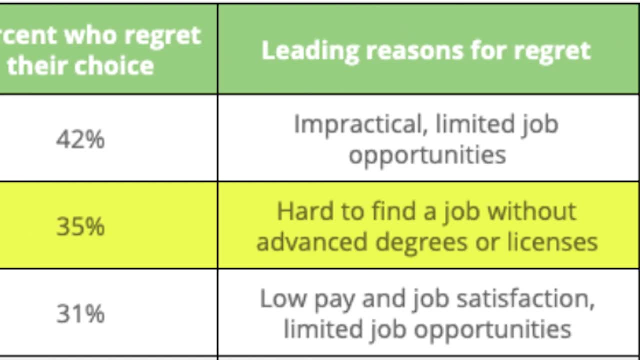 most regretted, in fact, at 35% of the people who get their degrees regretting them, according to ZipRecruiter- And the reason for that is because a lot of people expect to be able to get a job with just a bachelor's and unfortunately for many types of careers out there when it comes to science. 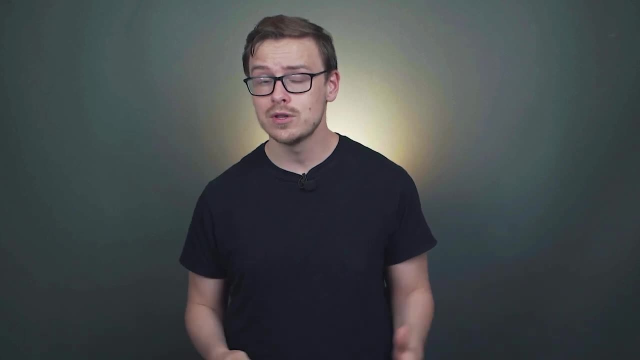 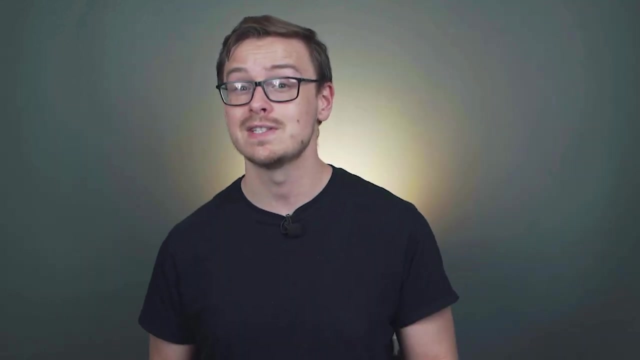 you have to get a master's or a doctorate. However, chemistry is one of the better science degrees and overall I would say that science degrees- when you're actually able to get a job, you do seem to be relatively satisfied with the career. Now, this is extremely subjective, like I. 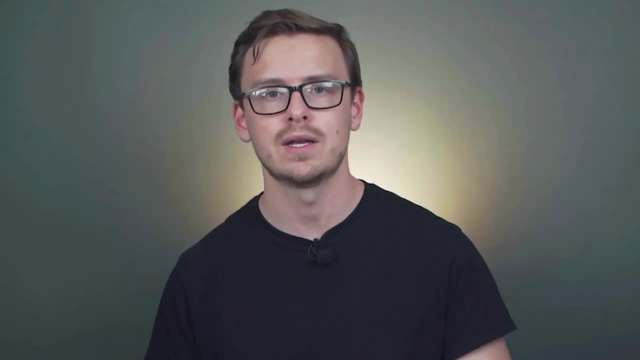 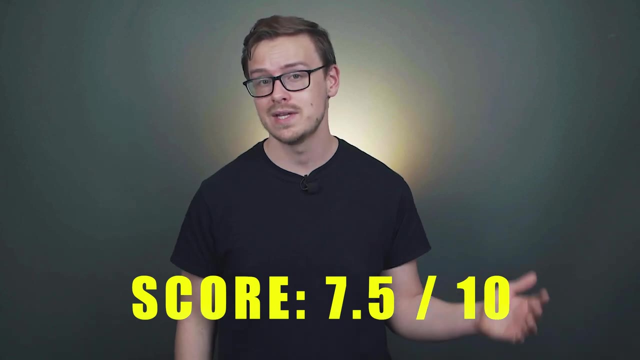 said, It depends on your personality. it depends on the industry you work in, what you're good at, company that you work for. in some cases, However, I'm going to go ahead and give this one a 7.5 out of 10.. Now, when it comes to demand, science related degrees are pretty average. for the most part, You 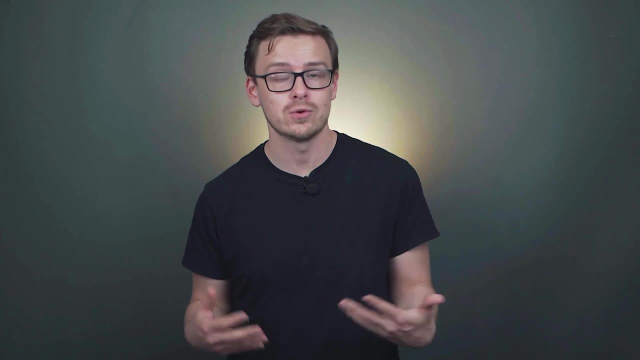 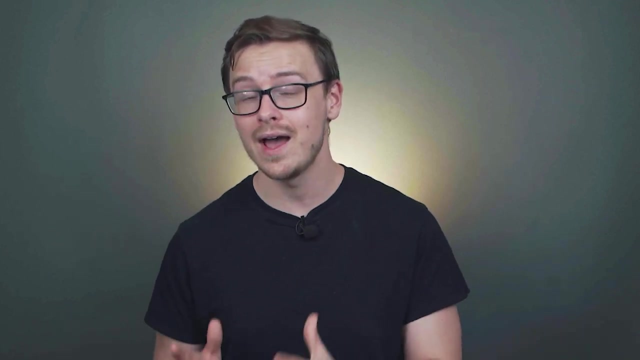 get a science related degree and then go into the health field, but that, of course, is going to be extra schooling. Health related degrees, health related careers, have the highest demand out of any type of career out there, even higher than technology. But let's say you're just sticking. 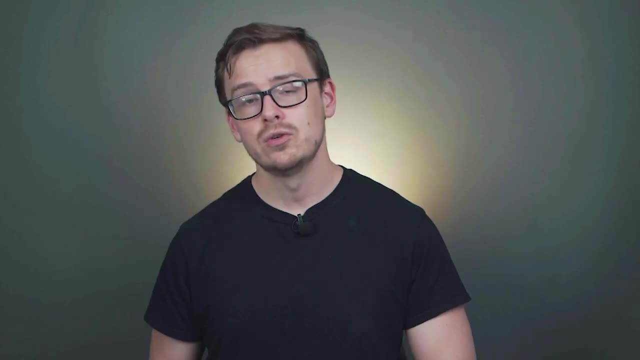 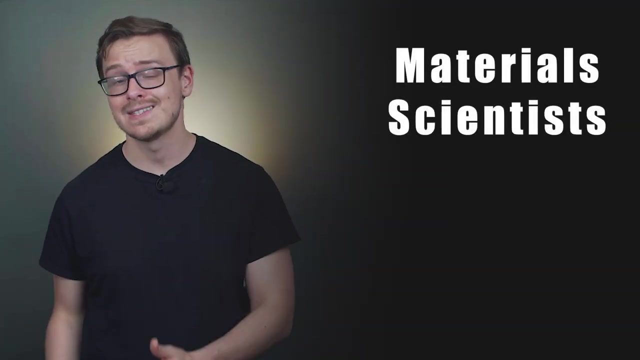 with a bachelor's and you're trying to get a job with just a four-year degree. So if you wanted to become a chemist, that one's growing at about five percent over the next 10 years. And if you wanted to become a material scientist, that one's growing at three percent, which is about average. Now if 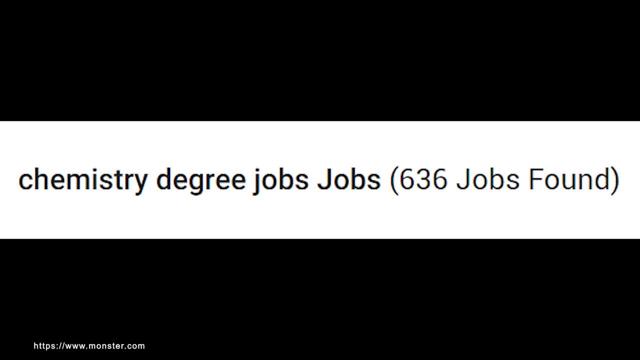 you search monstercom for the keyword chemistry, you're going to see that only around 600 jobs pop up. That means only 600 people had the keyword chemistry degree in their job listing. Compare that to computer science, which had 141,000,, and anthropology, which is around 800. 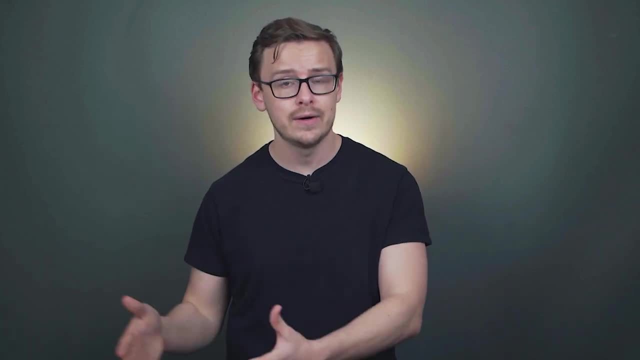 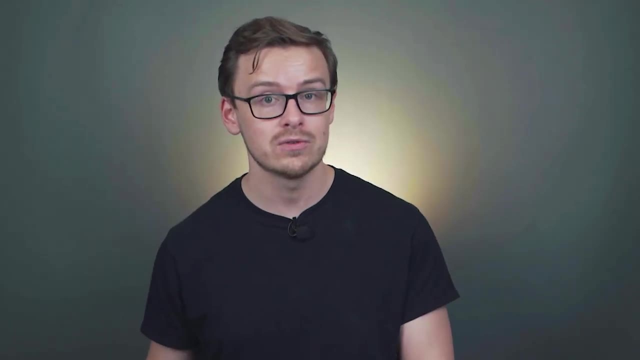 Now, it's not a perfect test by any means, but it gives me a hint that not a lot of hiring managers or owners are looking for people who have a chemistry degree. There's not an insane amount of demand out there, like computer science for instance, for people who have software development. 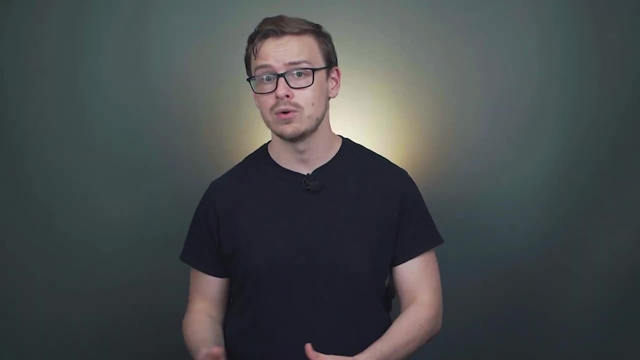 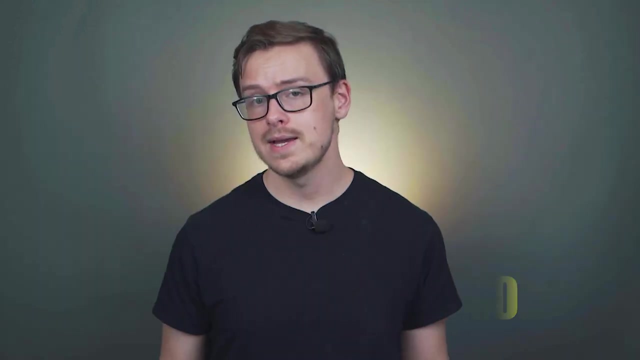 skills. Now, that doesn't necessarily mean that you won't get hired with a chemistry degree, but it is a little bit of a red flag. So with this one, I'm going to go ahead and give it a 6.5 out of 10.. Next we're going to be talking. 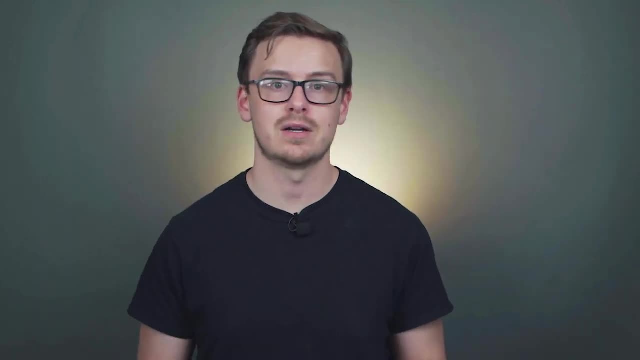 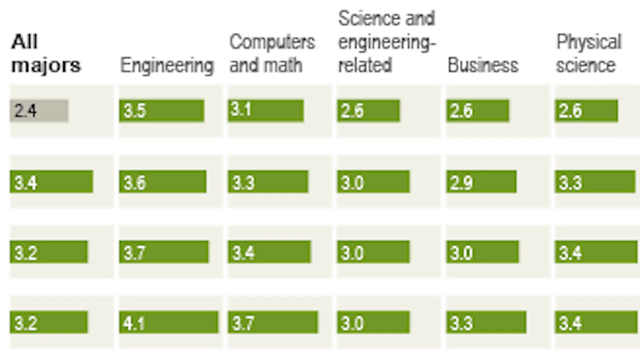 about x factors, which encompasses everything else that we didn't talk about already. So first, when it comes to physical science degrees like chemistry, they make around 2.6 million dollars over a lifetime, which is more than the average degree, which makes around 2.4 million. 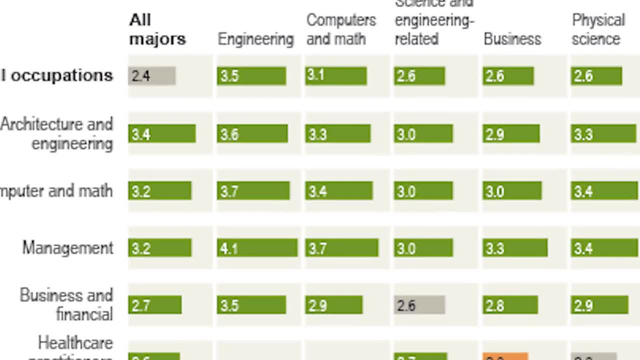 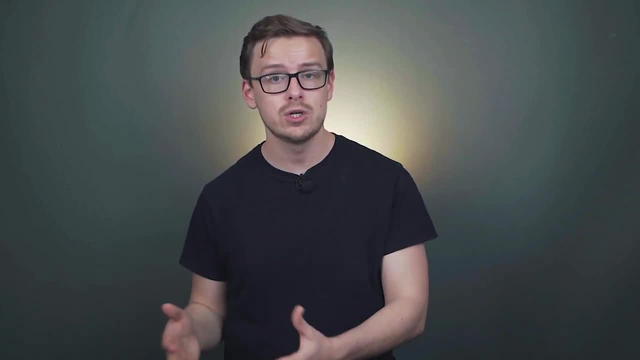 On top of that, you see that if they go into other career paths, like management for instance, they can make around 3.4 million over a lifetime. I think the reason for this is because if you're getting a chemistry degree, you're going to have a pretty strong background in science. 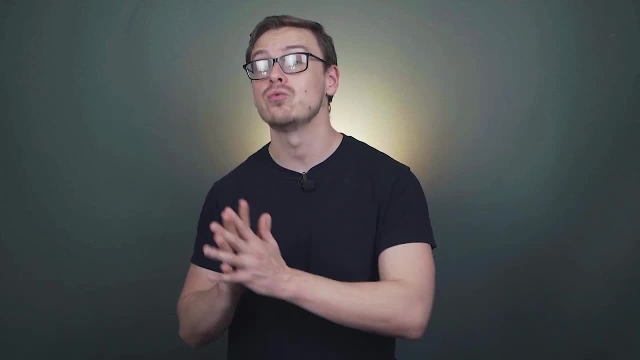 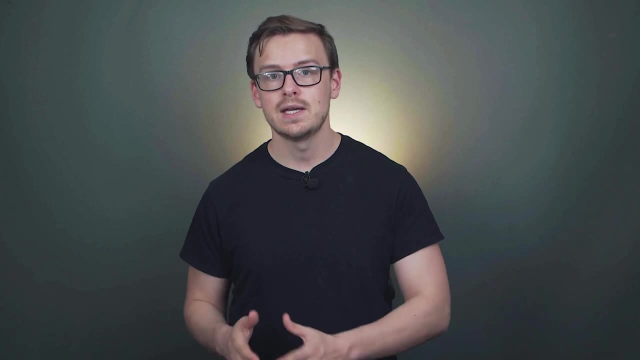 lab work and mathematics And, although that might not directly translate to helping you get a job, indirectly it's probably going to help you down the line. There's a lot to say with some of the hard skills, as well as some of the soft skills that you learn during college, indirectly helping. 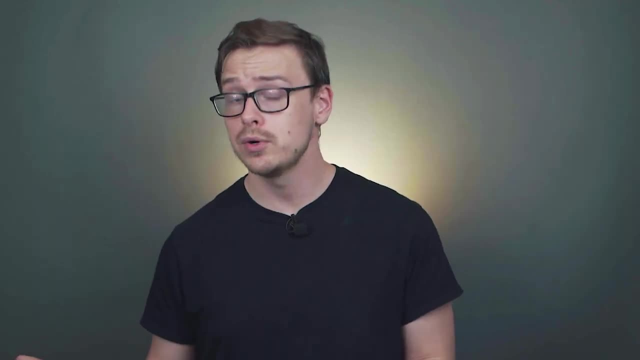 you throughout your entire life, And it looks like physical science degrees are pretty good all across the board. Now, when it comes to the skills that you learn, chemistry as a skill is rated 56 out of 100. So you're going to have to be a little bit more careful about what you're. going to be doing. You're going to have to be a little bit more careful about what you're going to be doing. You're going to have to be a little bit more careful about what you're going to be doing. on ZipRecruiter's skill index, Compare this to the highest rated skill of software engineering. 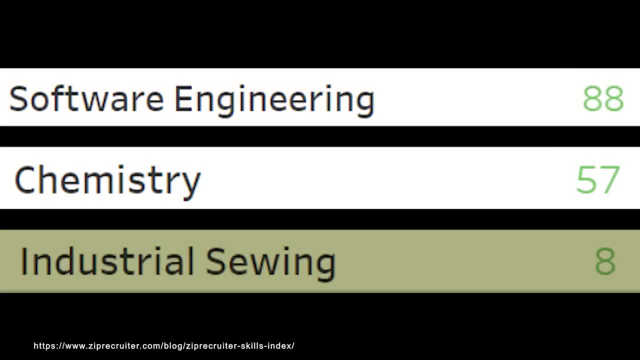 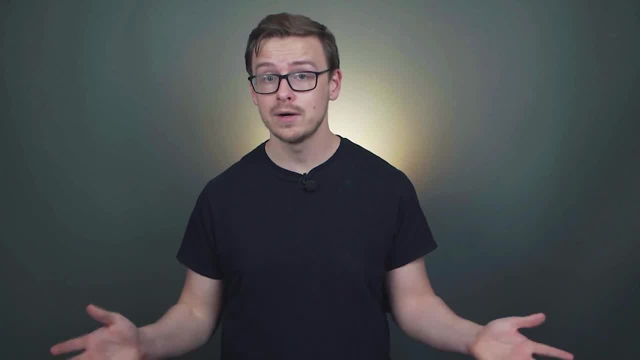 which is 88 out of 100, and the lowest rated, which is industrial sewing, at 8 out of 100. So it's going to be somewhere in the middle there. So the skill of chemistry is somewhat valued on the market. That doesn't mean that it doesn't have more value or less value than anything. 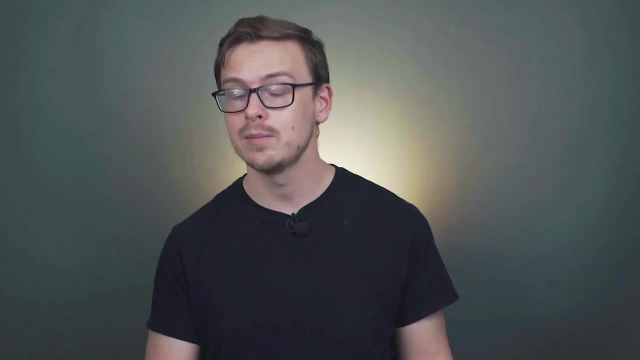 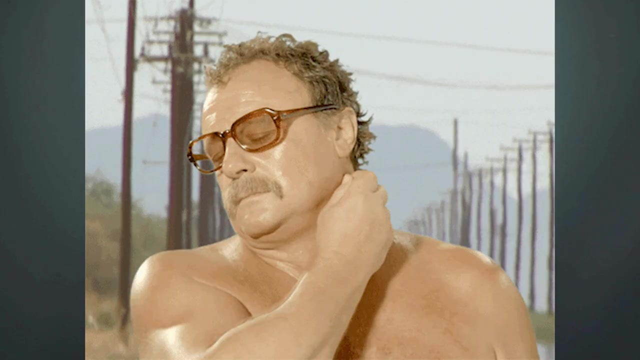 else. It simply means that people who own businesses and hiring managers are more likely to hire you and pay you more money if you have the skill of chemistry- Because, for whatever reason, it's pretty hot right now. You know, maybe 100 years ago industrial sewing would have been the 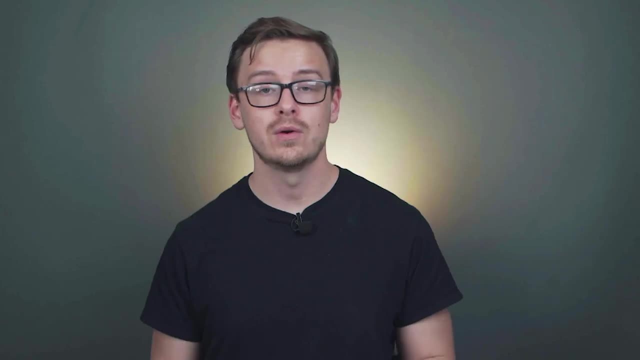 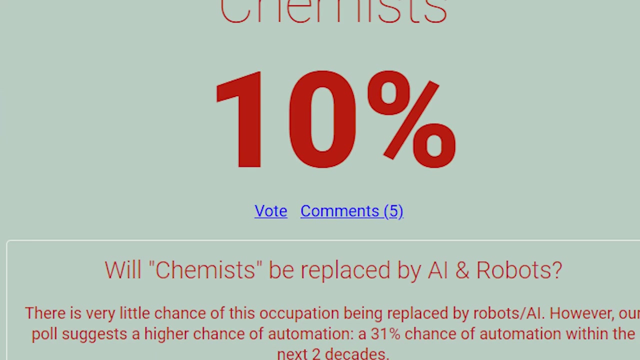 hottest skill around, but unfortunately, right now it's not really needed. Now, when it comes to automation, science degrees, science careers in general are relatively low, and chemists is no different. It only has around a 10% chance of being automated, And when it comes to difficulty, 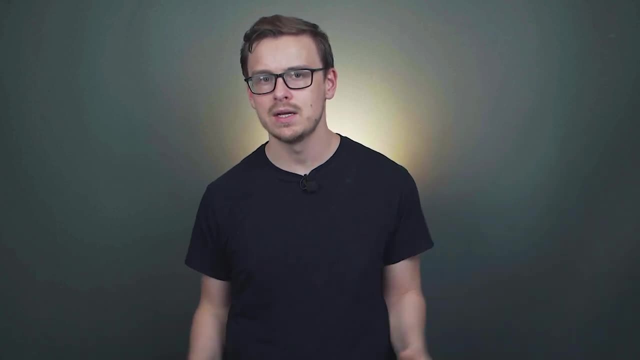 the science-related degrees are pretty high up there in my opinion, but they're probably not some of the hardest ones, except for physics. That one's really difficult, I think engineering degrees and mathematics degrees realistically are probably going to be harder for the average. 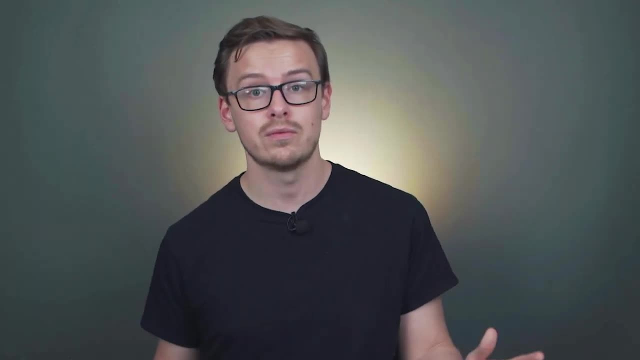 person. But again, that's extremely subjective. It could be completely different depending on who you are. You know, I took a lot of chemistry classes in undergrad. Organic chemistry is really difficult, Physical chemistry really difficult as well. I'm sure some of those upper chemistry 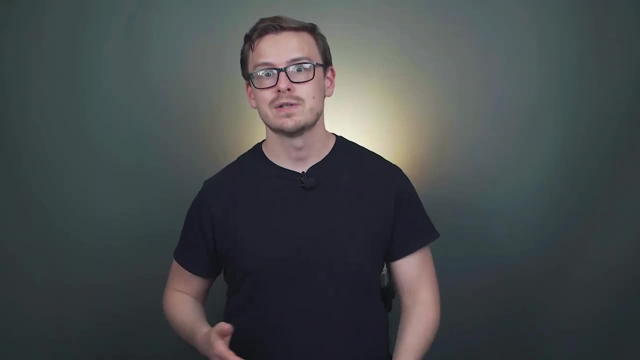 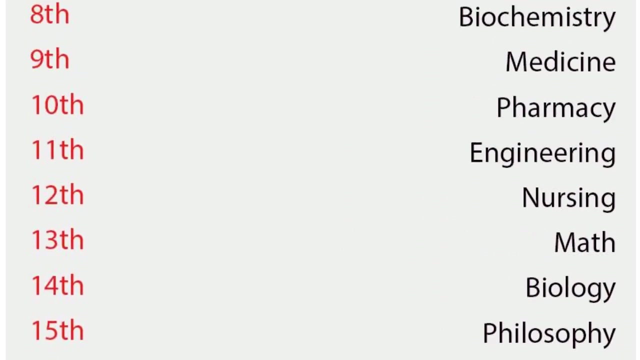 level classes get even harder, but I don't think it's going to be as hard as something like engineering. For what it's worth the reference I always use. tabcom, which kind of goes off of the dropout rate for the different majors, says that chemistry is the third highest. 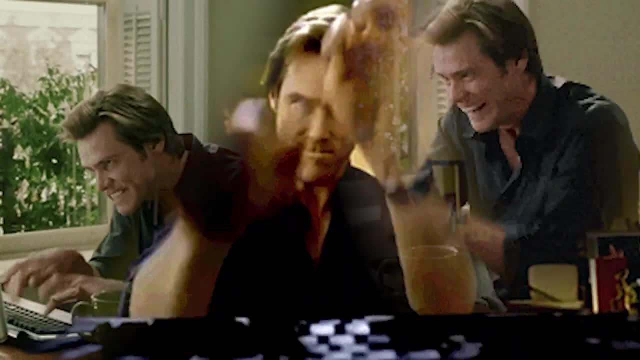 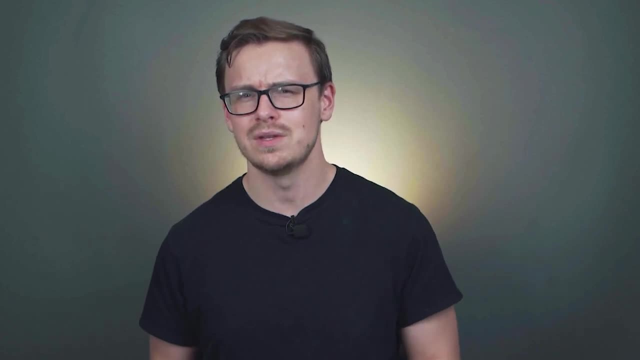 Let me know down below, if you're a chemistry major, how difficult it was. I mean, I'm not trying to say that it's easy or anything by that, by any means, but I didn't remember thinking that it was one of the hardest majors. but hey, maybe I'm wrong. But anyways, when it comes to flexibility, 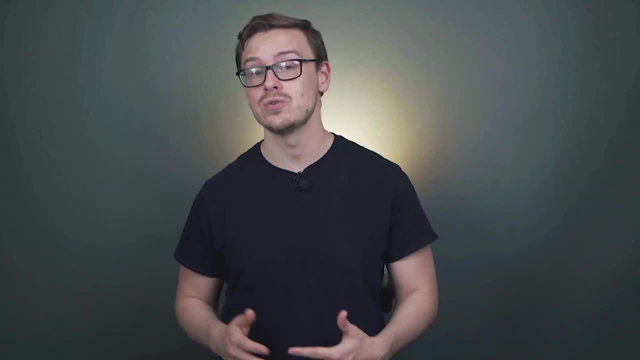 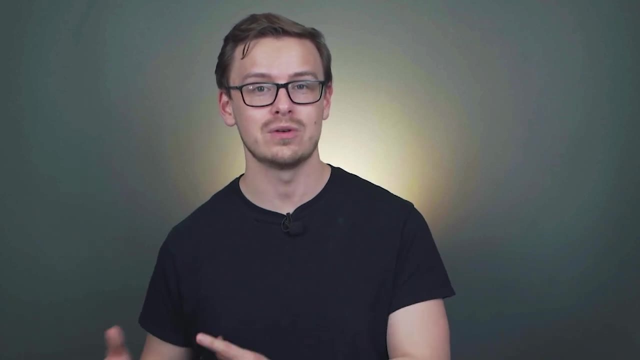 unfortunately, this is where some of the science degrees kind of don't do so well. For one out of all the different types of degrees, science degrees kind of make the worst combination with other degrees. So there's some types of degrees where if you double major in something else, 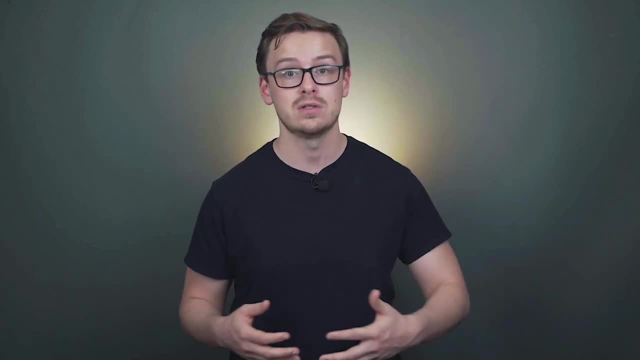 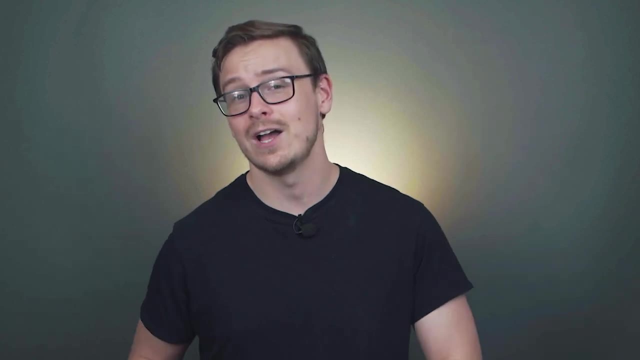 you know, it might not be that great on its own, but if you double major you can actually, you know, make it work With science related degrees. I mean, I guess it depends on what career path you're going down, but double majoring in something else isn't going to help nearly as 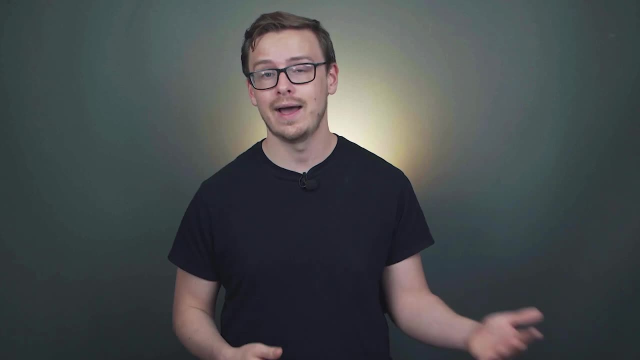 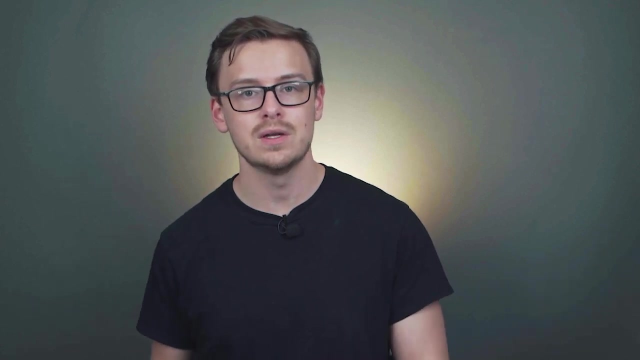 much, And when it comes to flexibility, they're honestly not that good either. A lot of the skills that you're going to learn are going to be relatively narrow. They're not going to extrapolate out to other things nearly as well as something like business, for instance, And so that makes